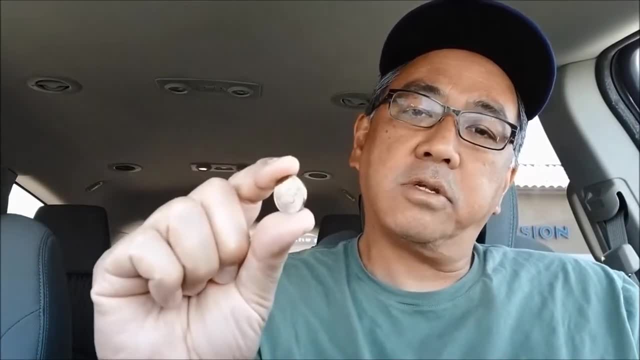 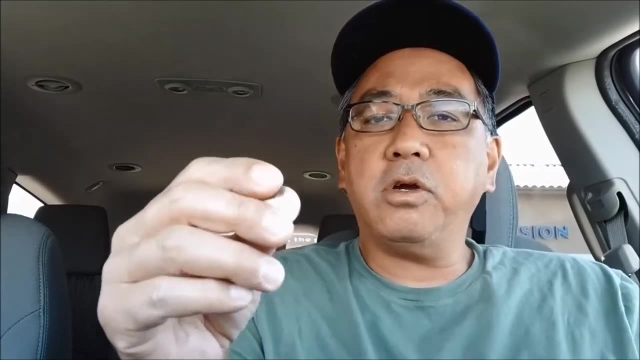 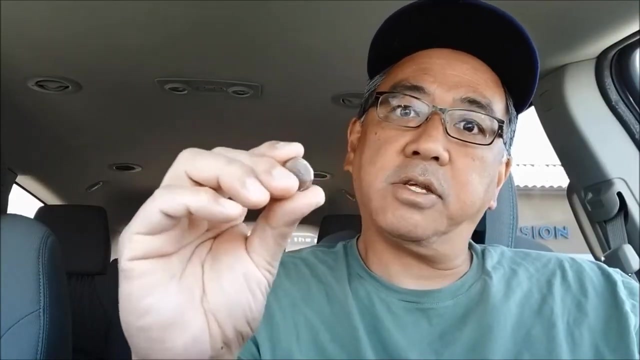 what do you think it's going to end up being heads or tails. And then what we want to do is use this as an experiment to find out: is it really 50%? So what you're going to do is you're going to just number from 1 to 10, put heads, tails, you know, whatever random outcome you think is going. 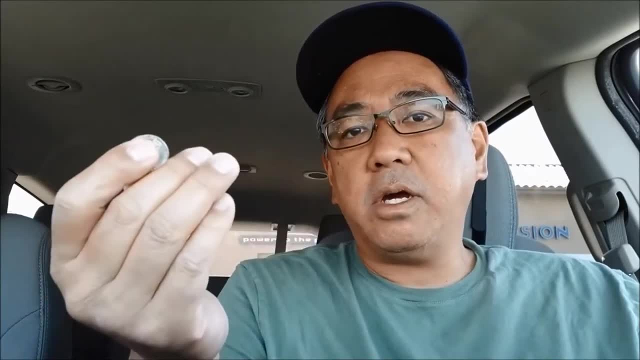 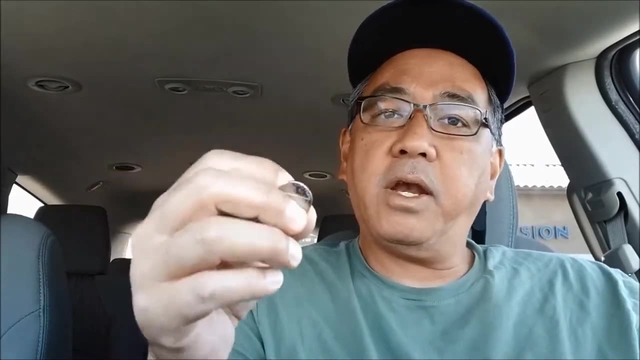 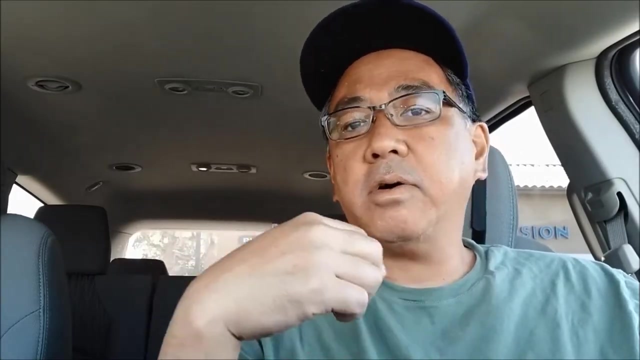 to happen from flipping a coin. What I'm going to do is I'm going to use Google- There's actually a heads and tails random coin flipper- and then we'll find out how you did. So I'll go ahead and start it off. I'll show you what I'm picking. I'll go ahead and do the random coin flipping. 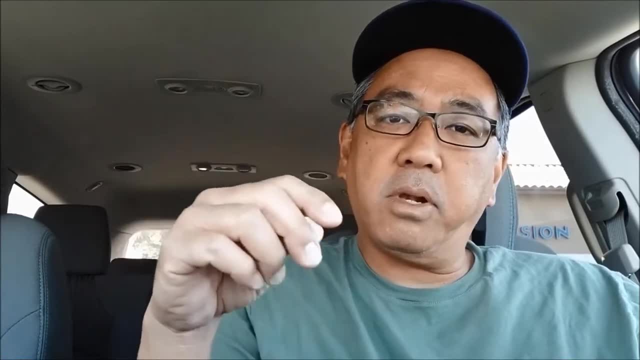 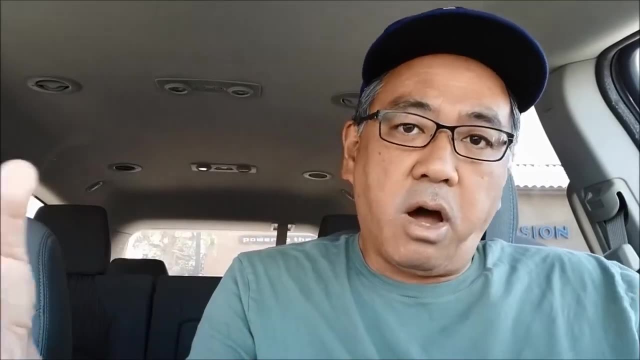 and then what I want you to do is, in the comment section down below, tell me how many did you get correct, and I'll do the same thing. What I plan to do is to you know, take all of your answers, put it together and see how close to 50% we actually get. 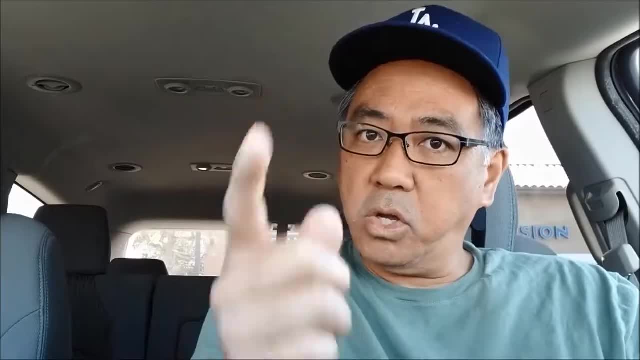 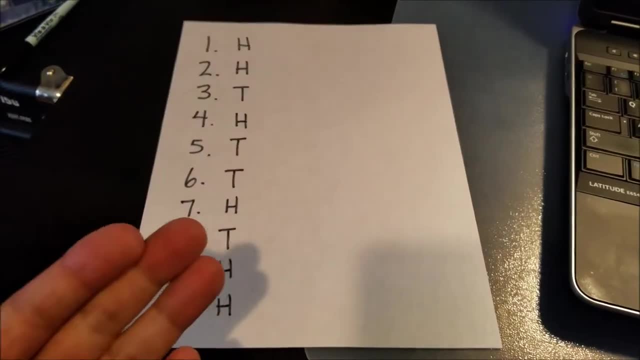 All right, Are you guys ready to do this? Okay, Ready set go. Okay, everybody. So here's all you do. You number, like I said, 1 to 10, and you just write down H for heads, T for tails, And what do you think is going to come up. 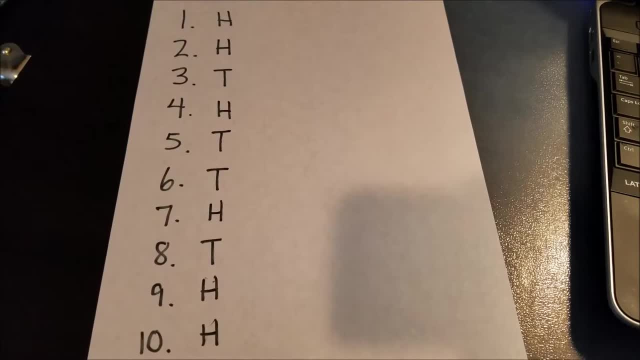 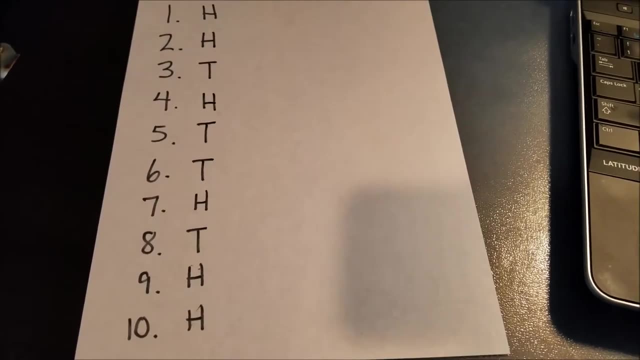 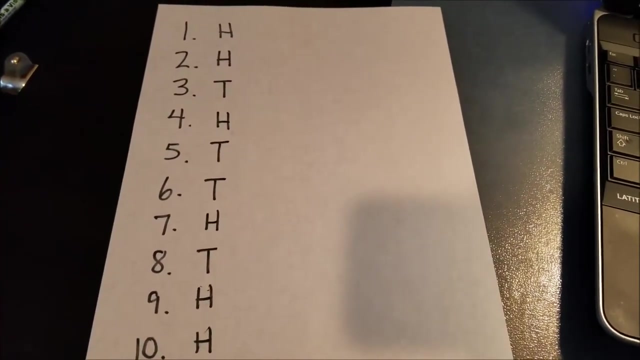 as I go through the random coin flipper. So I'm just kind of showing you what I did and I'm going to go to the random coin flipper and see how many I get correct. So one more time, Do the same thing and when I go over the random coin flipper, just mark off what you got wrong. 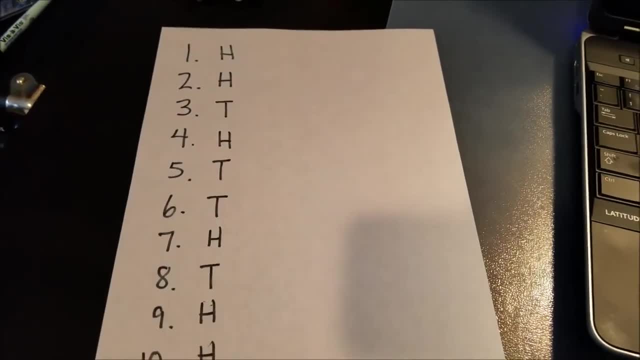 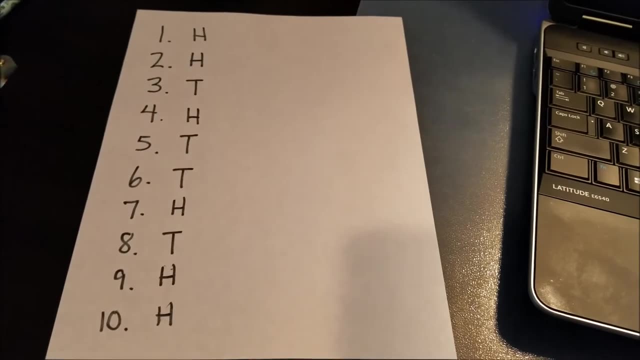 circle what you got right, or however you want to do it, but don't forget to tell me in the comment section how many did you get correct, because I'm going to use that data to kind of basically to show us how close to 50% we're all getting okay. 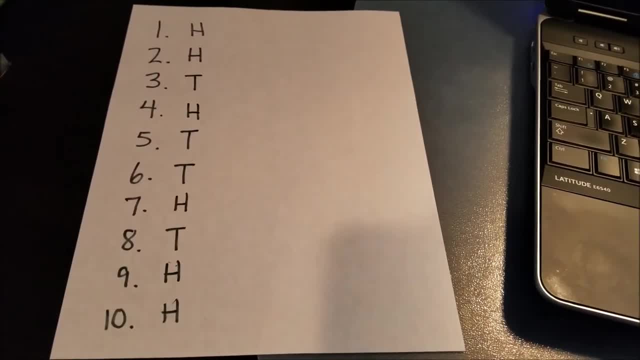 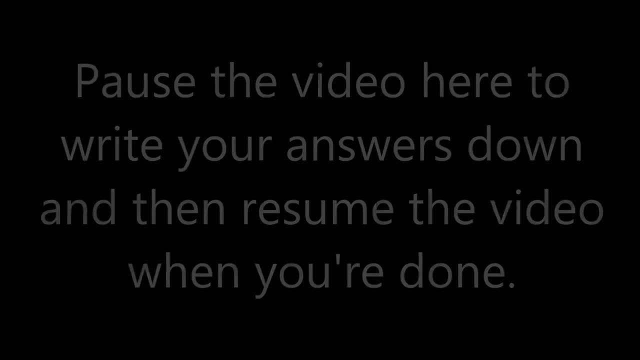 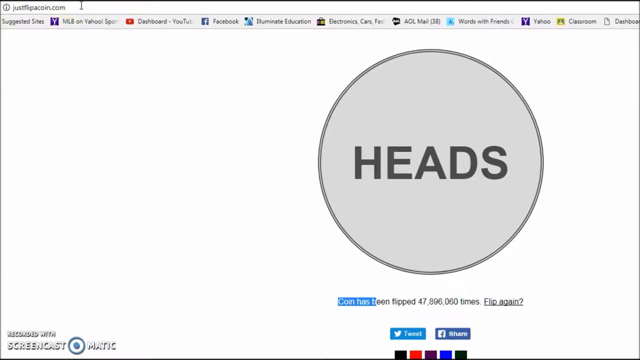 All right, guys, I'll go right now to the random coin flipper. Okay, guys, In the upper left here I just went to justflipacoincom in case you're wondering how I got to this, And I'm going to basically just click right here.